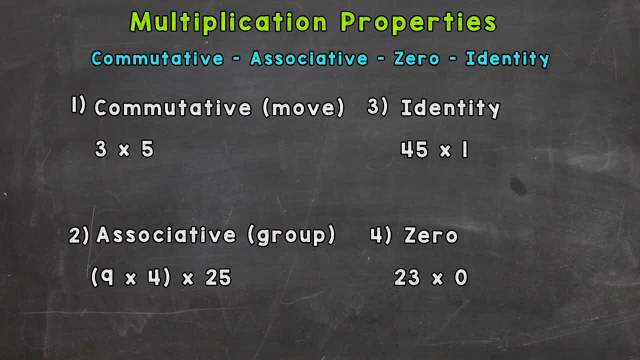 commutative property. you need to think, move. And our example problem: three times five gives us a product or answer of 15.. Now, commutative means that we can move these factors. The factors are the numbers that we multiplied together. We can move them and still get the same answer. So three. 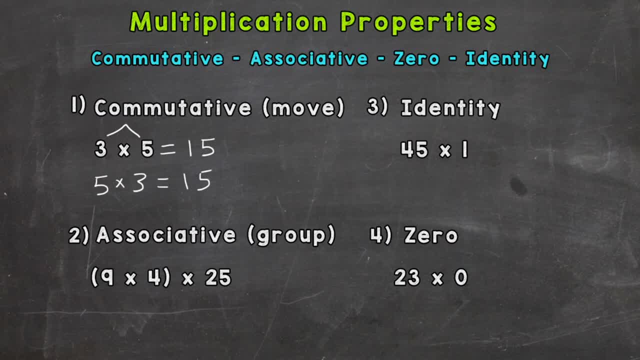 times five equals 15.. Five times three Also equals 15.. So commutative think move, Now associative, number two think group. So we have nine times four times 25.. And we have the nine and the four grouped here, So the parentheses in. 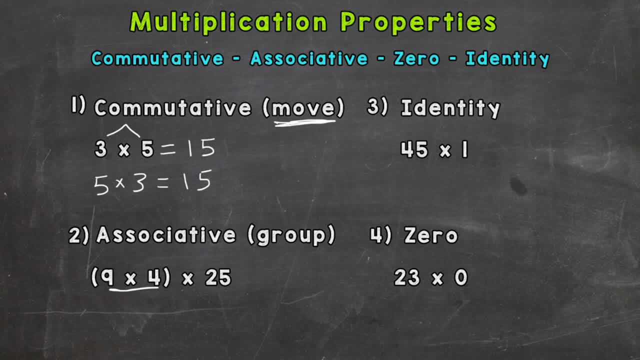 that problem means we need to do that first. So we would have: nine times four is 36.. And then we would need to multiply. So we would multiply that 36 by 25 to give us our answer. Now the associative property can make that. 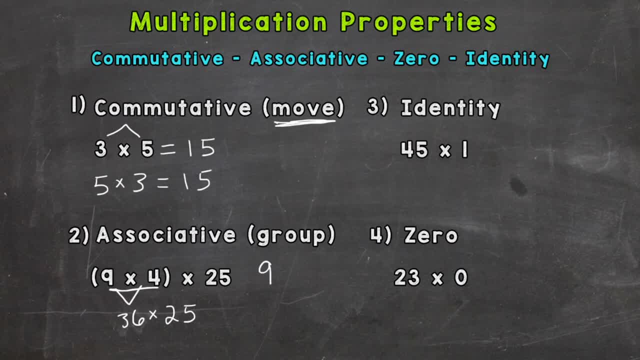 problem easier for us. What if we grouped the four and the 25 and did that part of the problem first? Well, four times 25 is 100.. Bring down our multiplication sign and the nine, And now we have a nice and easy mental math problem. 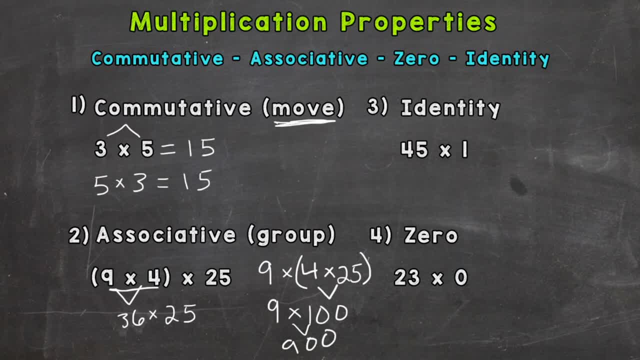 Nine times 100 is going to give us 900.. 36 times 25 is also going to give us 900.. But which problem was able to be solved easier? Well, when we grouped the 4 and the 25, because we could use mental math strategies to solve that. 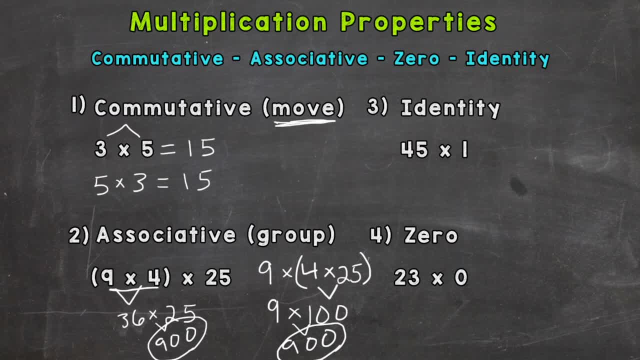 So associative think group Now 3, we have the identity property of multiplication, And the identity property states that anything times 1 is that number itself. So 45 times 1 is going to give us 45. If we did 78 times 1, that would give us 78.. 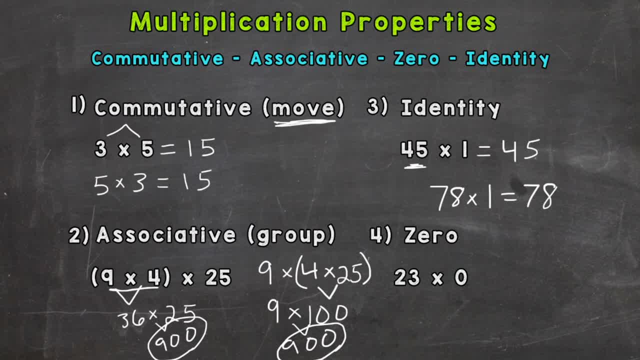 So anything multiplied by 1 gives us that number itself. And then the last property we're going to discuss is the 0 property, And that states that anything multiplied by 0 equals 0. Whether it's 23 times 0, 1000 times 0, 72 times 0, anything times 0 equals 0.. 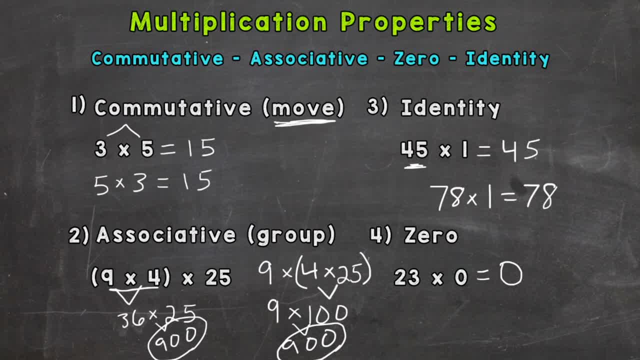 So there you have it. Those are the 4 multiplication properties that we wanted to cover in this video. I also have a video on the distributive property. If you want to check that out, I'll put the link down in the description. 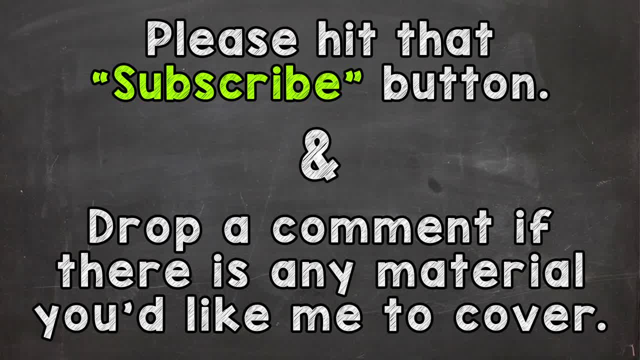 Thanks so much for watching. Until next time, peace. 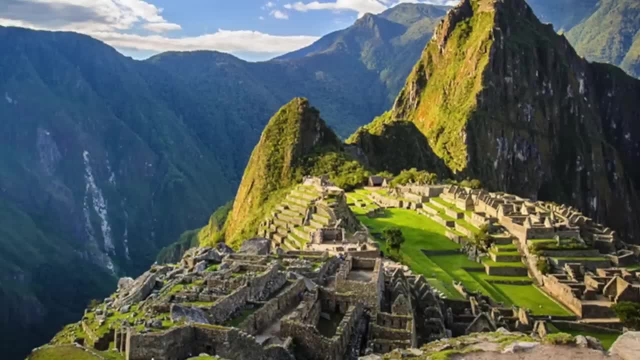 Okay, so you've probably heard of Peru. This is a popular one. You know llamas, machu picchu, ceviche, the Incans- But what you probably don't see too often is the larger scope of what Peru has become in modern times. 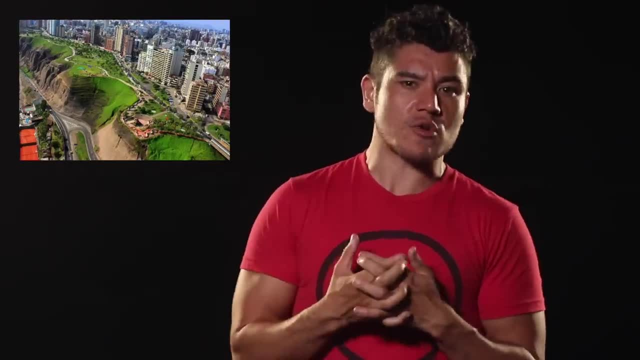 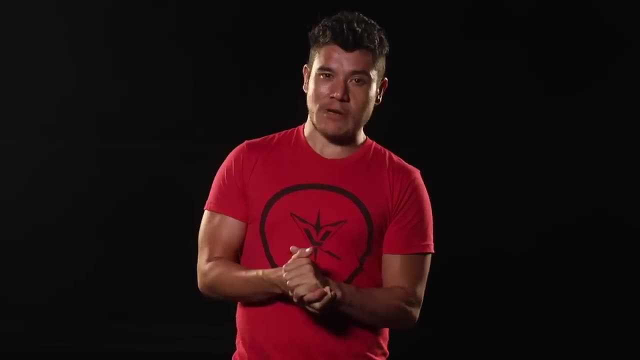 It's this desert-y, mountain-y, jungle-y, Asian-fused West Coast business-oriented chef of the Latin world. Yeah, chef, No one cooks like Peruvians And they'll Peruve it to you. Yeah, there you go. That's my pun for the episode. 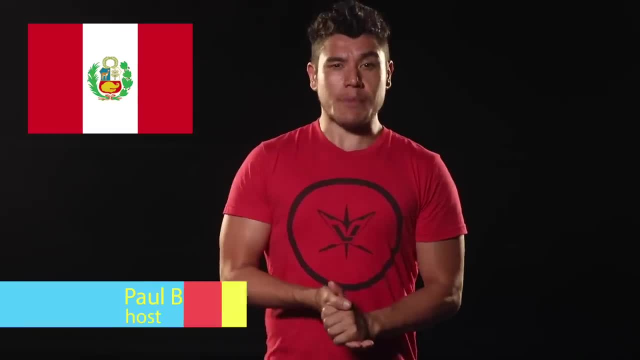 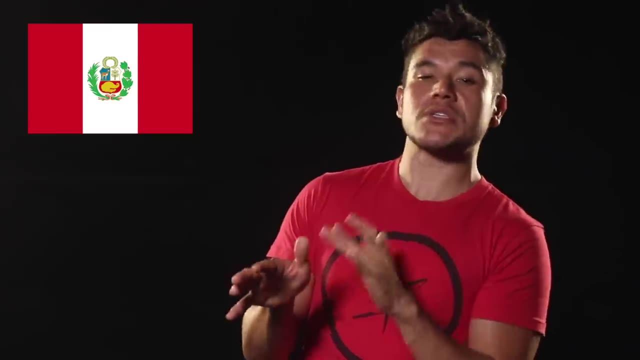 It's time to learn geography. No, Hey everyone, I'm your host, Barbs GeographyPoop. Jorge Carlos says Peru is a beggar sitting on a gold bench. There's lots of stuff to deal with, yet so many riches they have. 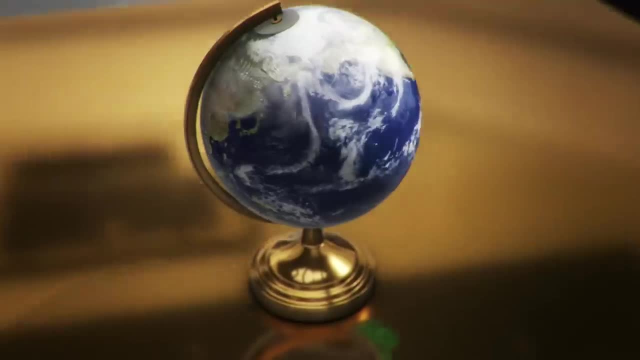 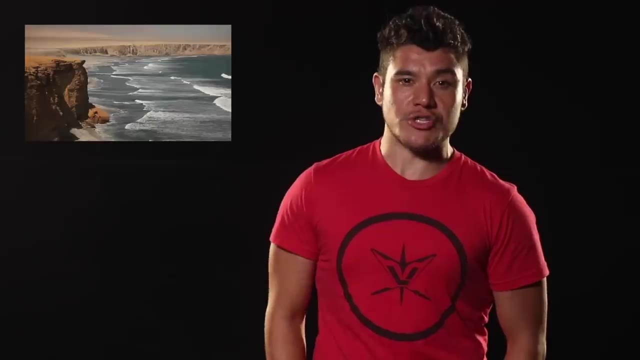 And now it's time to open the treasure map and find the pot of gold, shall we? In South America, location matters. Everybody wants two things: resources and ocean Shut up, And if you can have both, plus some really cool straw hats, you're probably gonna do well. 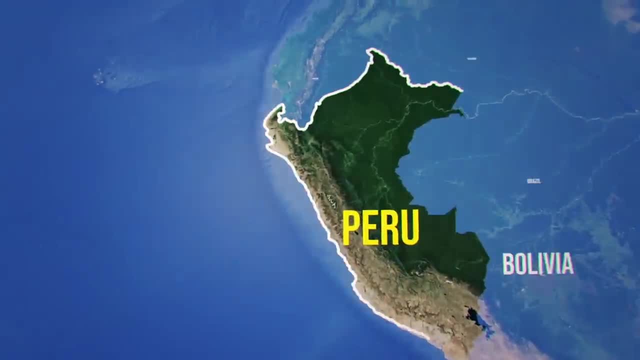 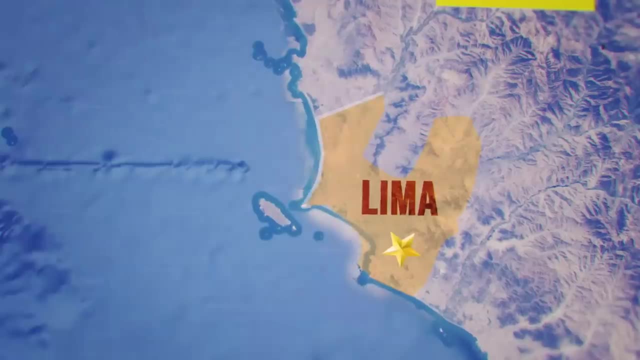 First of all, the country is located on the west coast of South America, bordered by five countries. The nation is further divided into 24 states, Each with their own flag and seal. The capital and largest city of the country is Lima, which also acts as its own department. 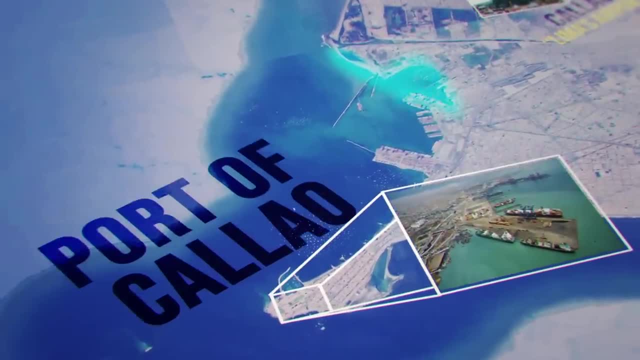 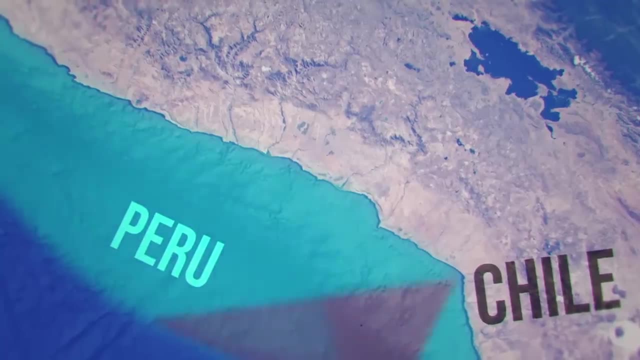 Just a skip away, you can also find the largest and busiest shipping port, the Port of Cayo, where most major cargo ships dock and transport traded goods. Speaking of the coast Down at the bottom of Peru, they have a slight maritime dispute with Chile, which kind of looks like this, but it doesn't really cause too much trouble.